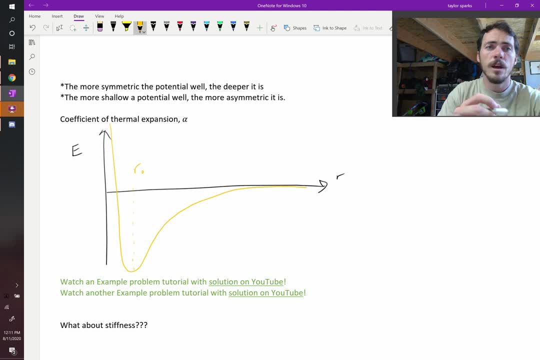 It's not going to be vibrating anymore. It's just going to stop and it's going to stay put. And where will it be when it stays put? It's going to be right here. That's going to be where your atom lives at, your compound lives at. 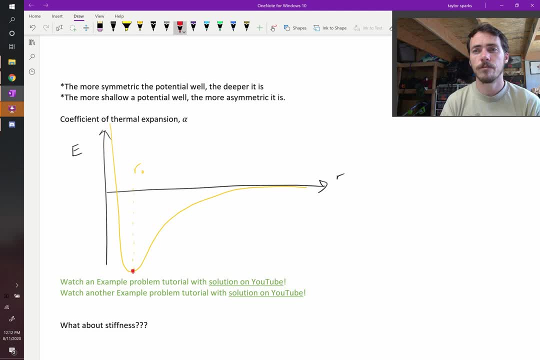 The bond distance is going to be exactly r-naught. But now imagine with me, if you will, what happens when we heat this thing up a little bit. If we heat it up just a little bit now, we're giving it thermal energy. 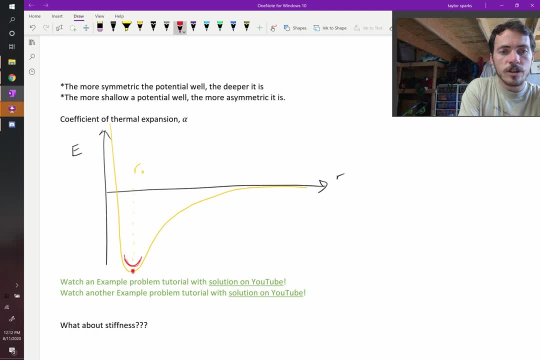 As we go further, we're going to see that it's going to be exactly r-naught To give it thermal energy. we're allowing it to slosh back and forth in this potential. well, We're allowing it to not just stay in the lowest. 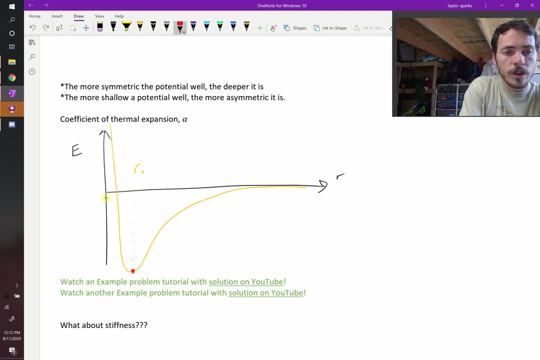 It has a little bit of energy so it can move around a little bit. So what we're really doing is we're giving it energy up to certain levels as we heat it up. And as we keep on heating this thing up, look what's happening. 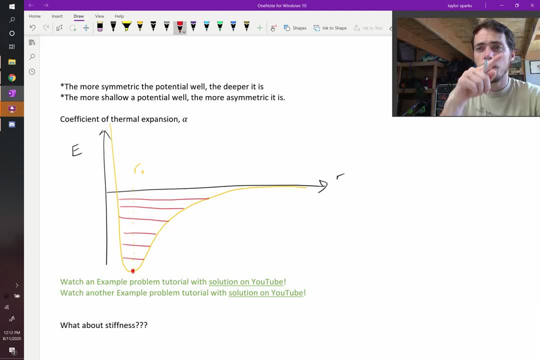 Where is the average position at any given time? We know it's sloshing back and forth in this. well, but where's the average position and what's it doing? Well, we can plot it. Let's draw the average position, the middle position. 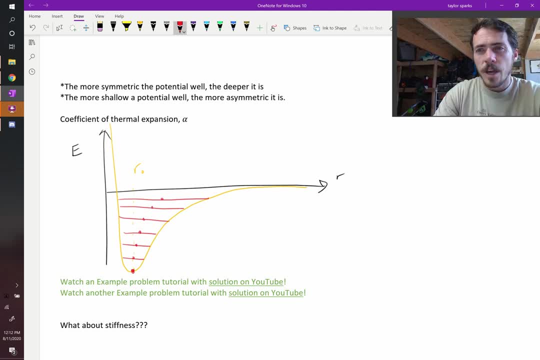 Check it out. What's happening to our average position as we heat it up? It's moving right. It's actually moving with us, typically outward. It's getting bigger. The molecule's expanding At absolute zero. your negative and your positive have some separation distance r-naught. 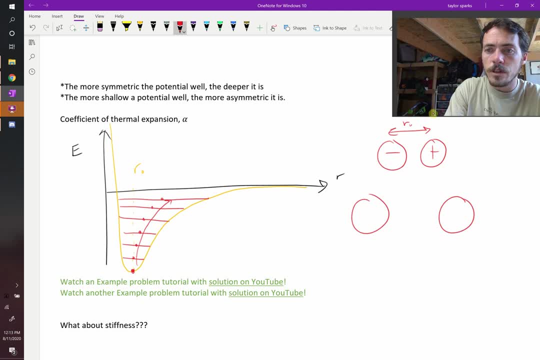 But as you heat this thing up, they're literally getting more separate from one another. So this r at high temperatures, we'll call it r-one And that could be maybe right there: r-one. They're getting more and more separate from one another. 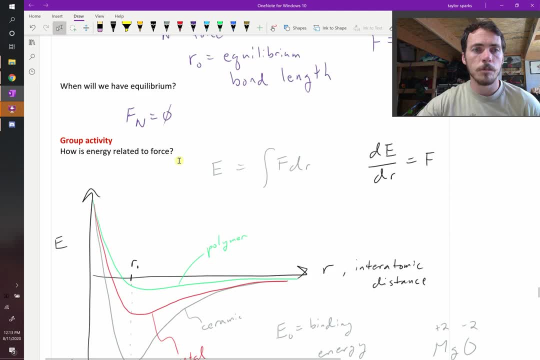 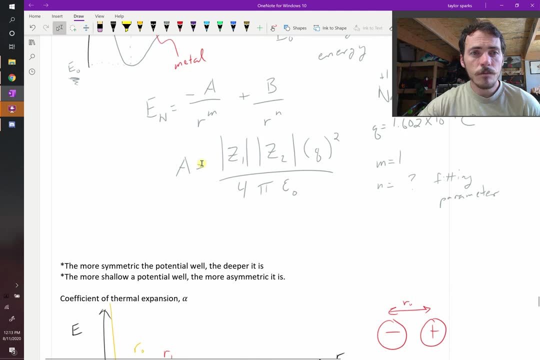 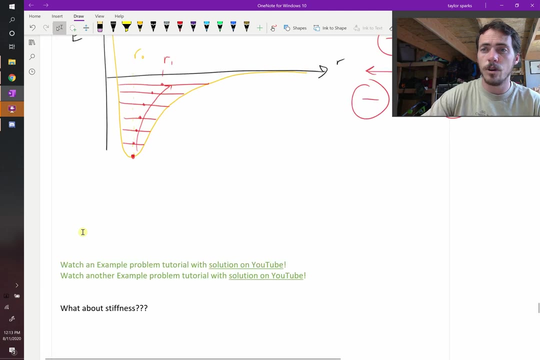 So these potential energy diagrams, if you had a way to plot them and you could look at the asymmetry, you could figure out the coefficient of thermal expansion, Because in some cases they might look like this, But in other cases let's picture like a polymer or a metal which doesn't go as deep. 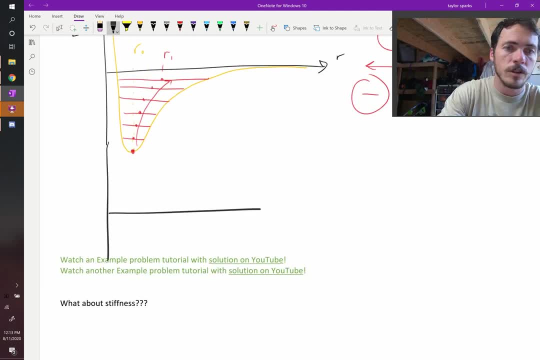 It might look like this. So let's draw this one over here. The polymer, or let's say it's a metal- It might do something like this. Well, now look what's happening. Here's its lowest point, And as you start to heat it up, its average position is increasing at a larger rate, right? 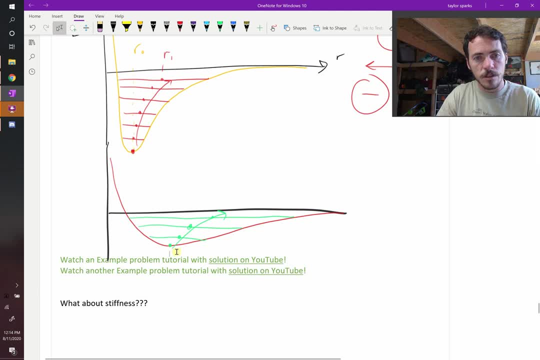 This is less rapid onset and this is more rapid. So polymers and metals are going to expand thermally more than ceramics. Ceramics are going to expand. They're going to expand the least. typically. Metals expand a little bit more. Polymers expand a lot more because they're the most shallow potential energy. well, 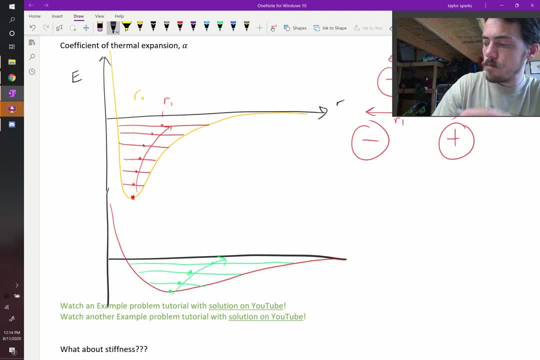 So we can actually write these things down. We can say that ceramics are typically 1 to 10 parts per million per Kelvin. That's how much they expand. So what are the parts per million? You know how we say percent, That's parts per 100.. 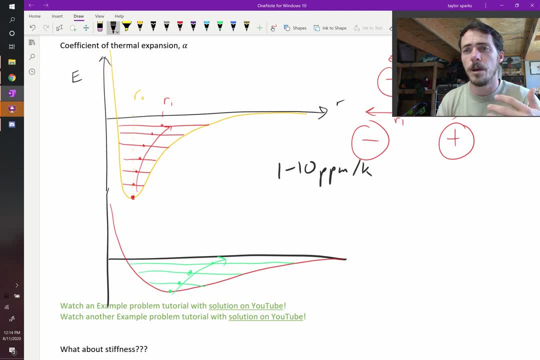 1 divided by 100.. So parts per million just means you take the number and you divide it by a million. That's all that means. And then per Kelvin. So for every 1 degree Kelvin that you heated up, it increases by whatever this amount is. 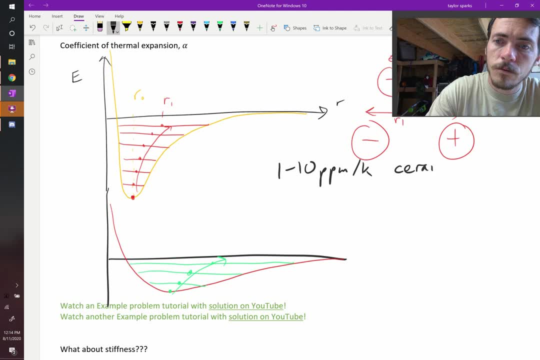 So those are your ceramics. A metal and a polymer are going to be greater than that. A metal is typically on the order of 10 to 100 parts per million per K- PPM per K- Whereas a polymer very often are greater than 100 PPM. 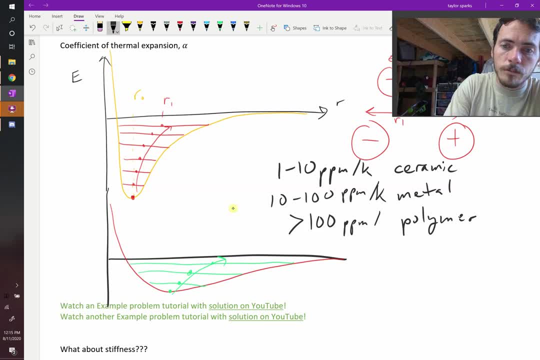 So this is a nice rule of thumb that holds. They're typically about this orders of magnitude, Like a ceramic is about 10 times less than a metal. A metal is about 10 times less than a polymer. So let me ask you this: 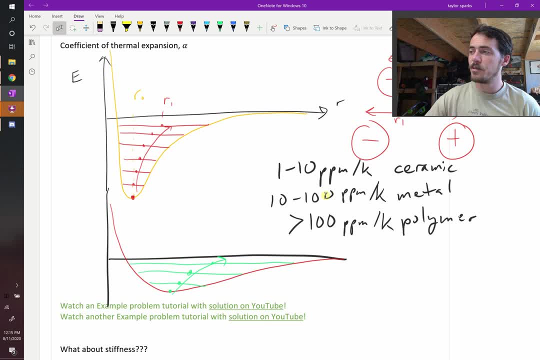 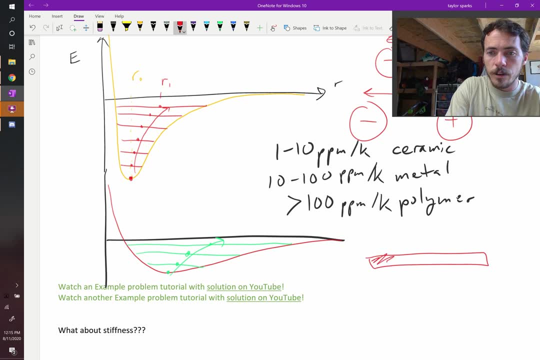 What's going to happen when you make some sort of device? right, You make some handy-dandy contraption for your next invention And it's made up of a polymer- right here, Sweet, Sweet polymer, And that is a polymer And that is bonded with some sort of strong epoxy or something to a metal.